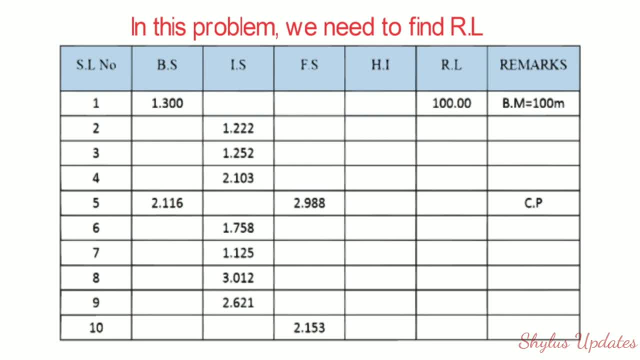 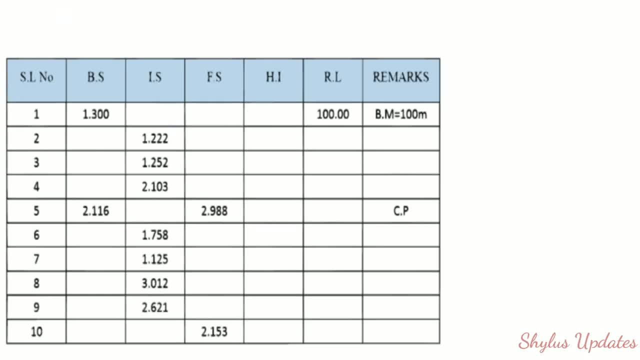 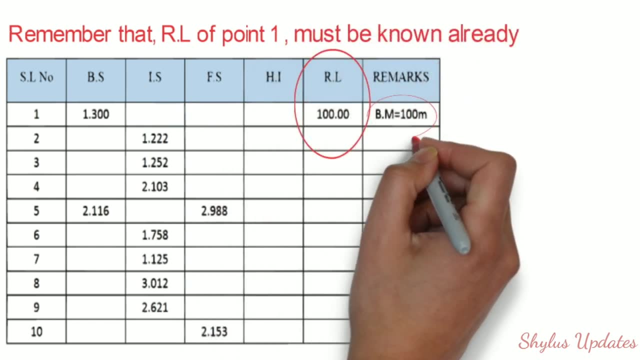 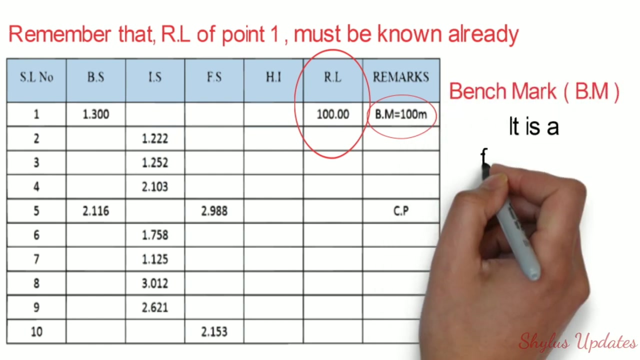 In this problem. we need to find reduced level of this ten points. Remember that reduced level of zero level must be known already, ie benchmark Benchmark is equal to 100 meters. What is mean by benchmark? It is a fixed point of reference of known elevation To calculate reduced level of these remaining. 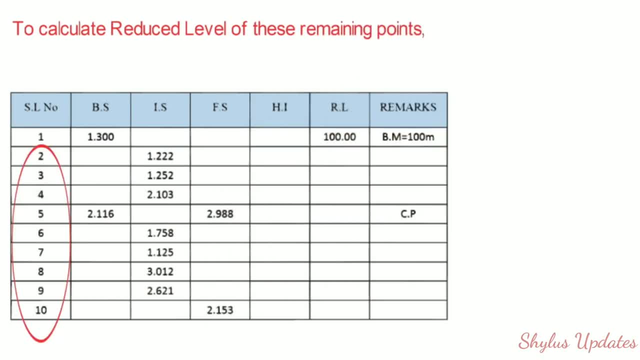 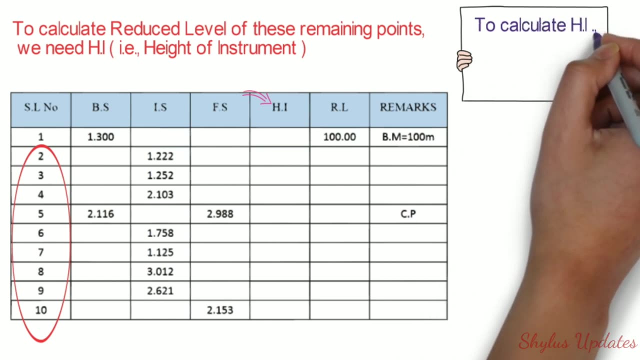 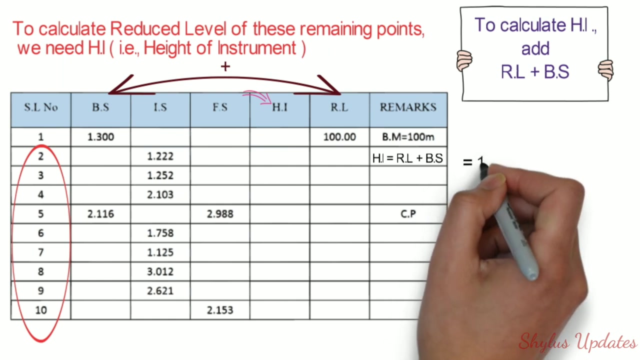 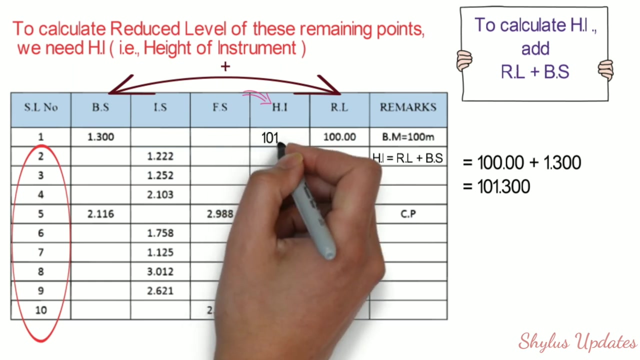 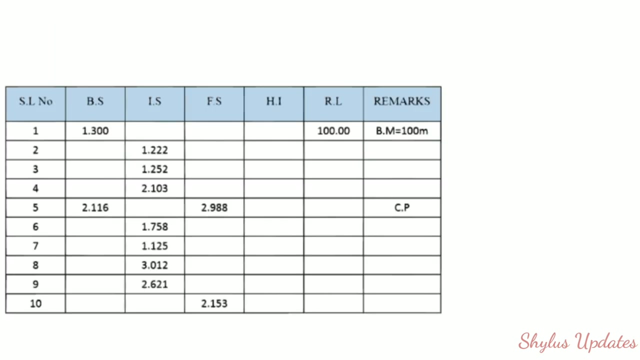 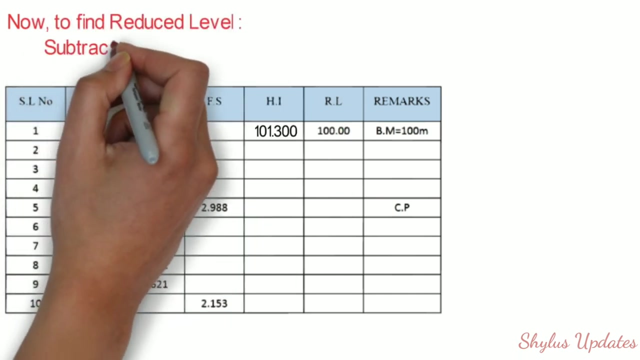 points ie from 2 to 10, we need HI ie height of instrument. To calculate HI, add reduced level plus back side, ie 100.00 plus 1.300 is equal to 101.300.. Now to find reduced level subtract intermediate. 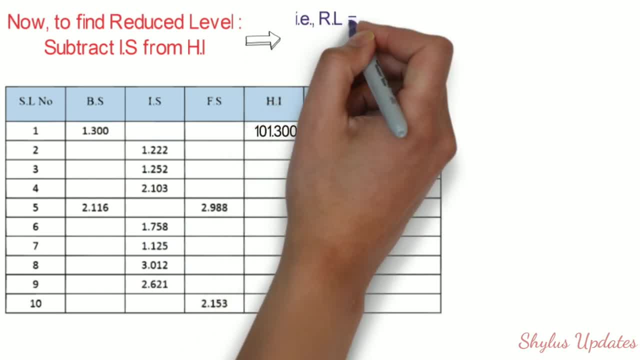 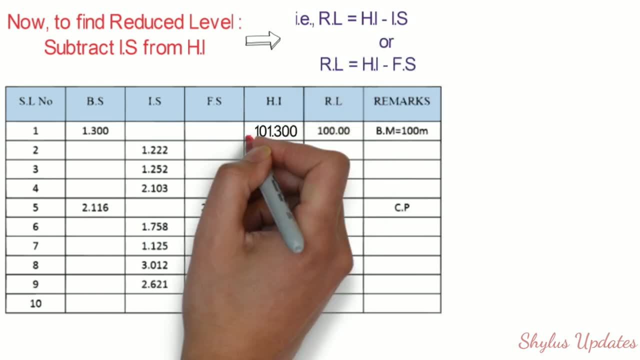 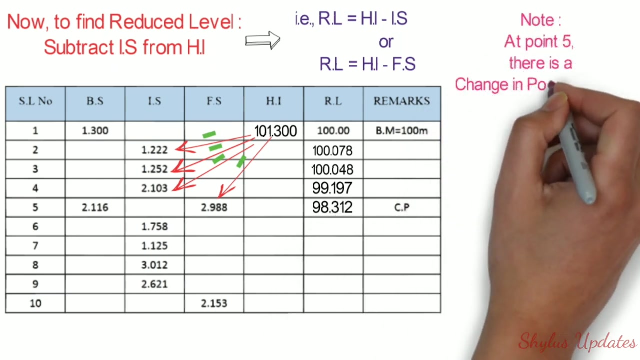 side from height of instrument. ie reduced level is equal to HI-IS or HI-FS. Note at point 5, there is a change in position of instrument. ie reduced level is equal to HI-IS or HI-FS. 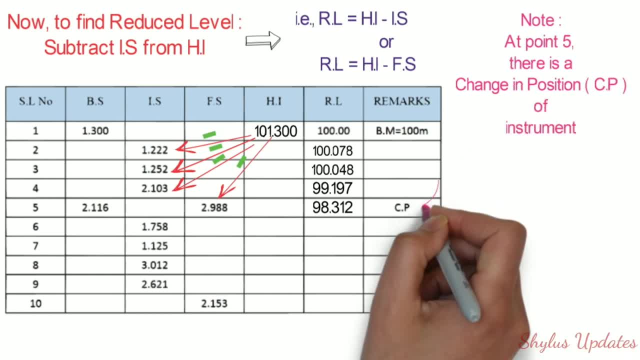 Note at point 5, there is a change in position of instrument Which I have mentioned in remarks. Now we have only reduced level and back side. This value is reduced level and this value is back side, Which means we have to find height of instrument again. We know that height of instrument is equal to the height.